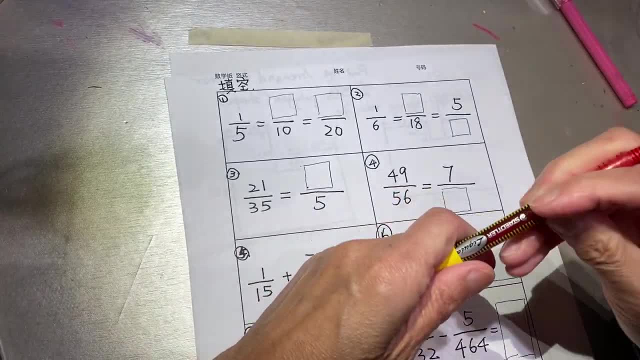 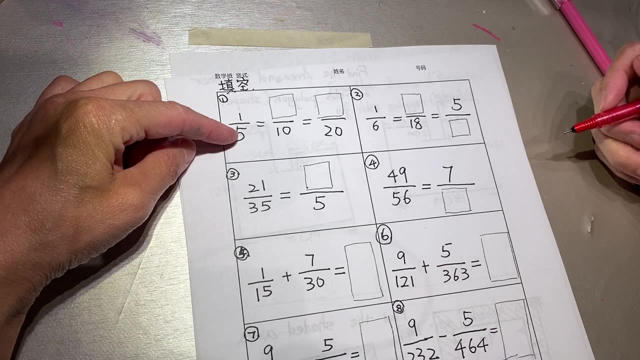 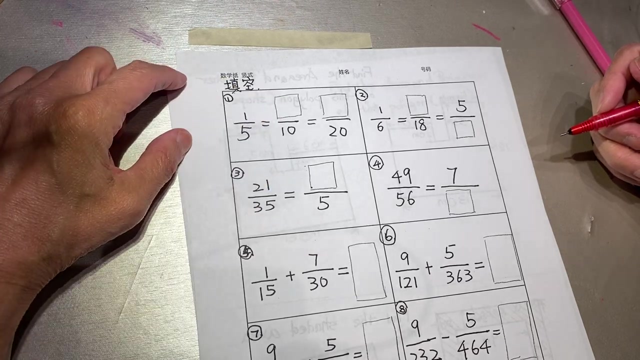 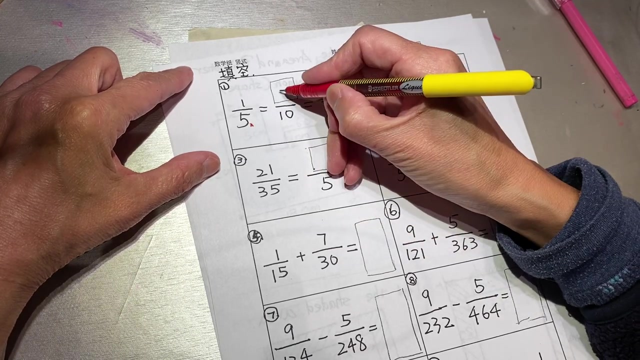 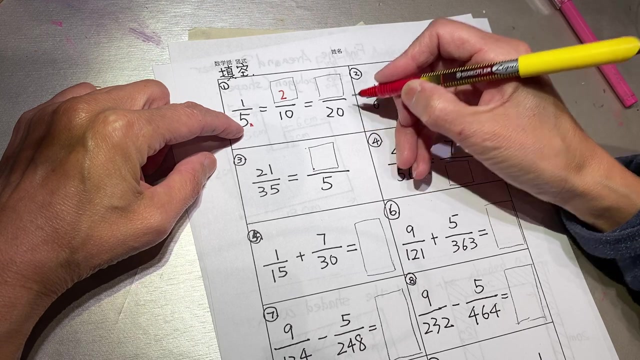 Okay, so the teacher does not know how to fill in the blank. We will help her. 1 over 5 equal to how many over 10?? So you can see. this is equivalent fraction Time. 2 becomes 10.. So 1 times 2.. 5 times 4 is 20.. 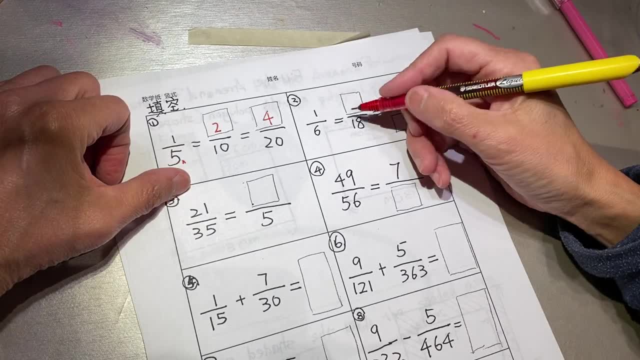 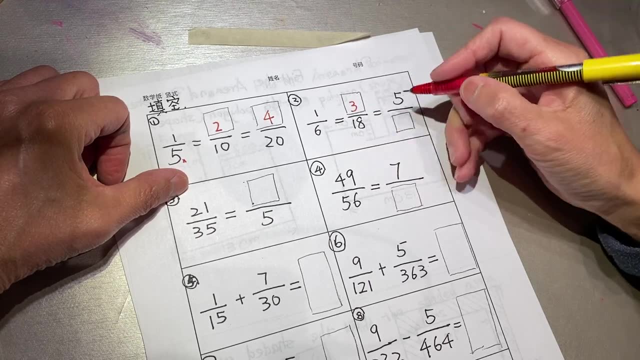 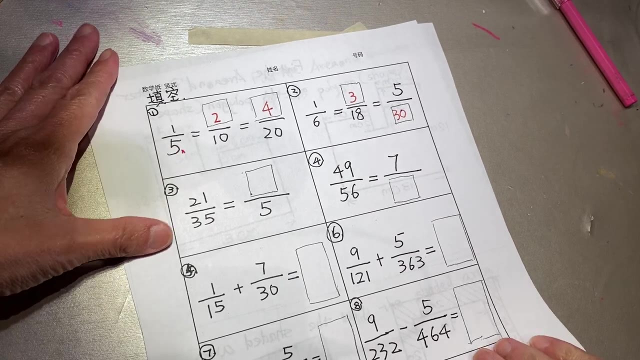 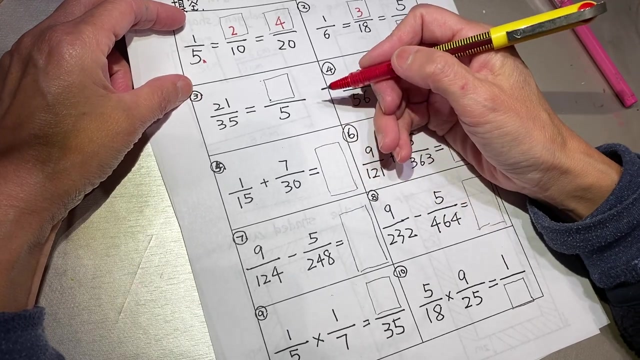 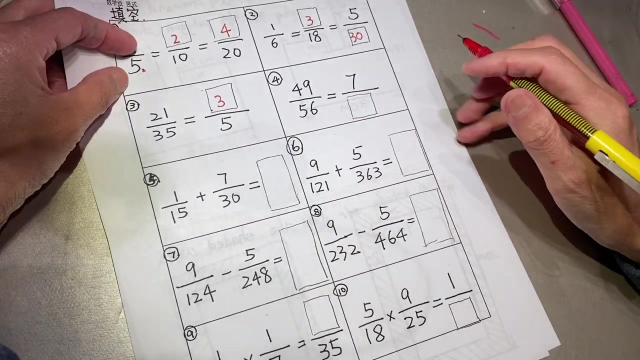 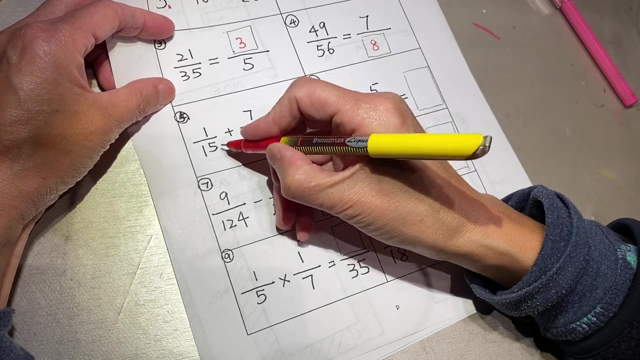 Question number 2,, 1,, 6,, 3,, 8, and 13.. And this seems to simplify an equivalent fraction Divided by 7.. Divided by 7.. Divided by 7.. 8. Time 2.. Time 2.. 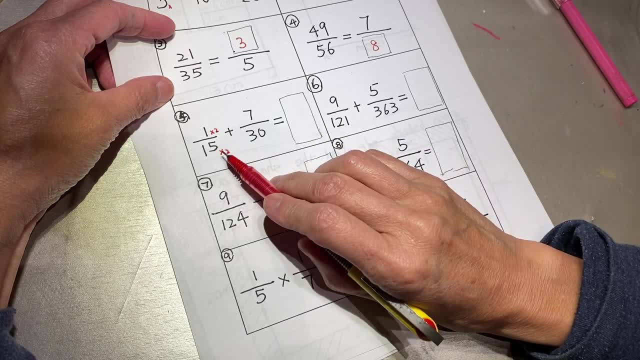 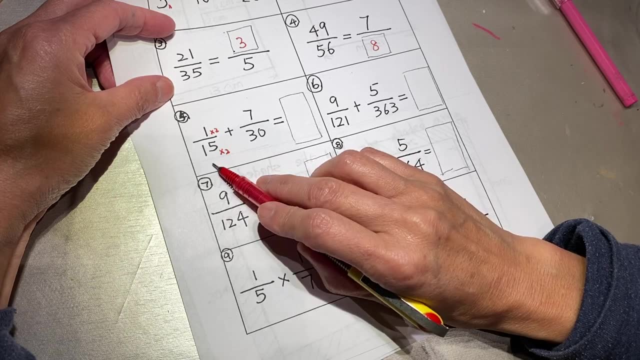 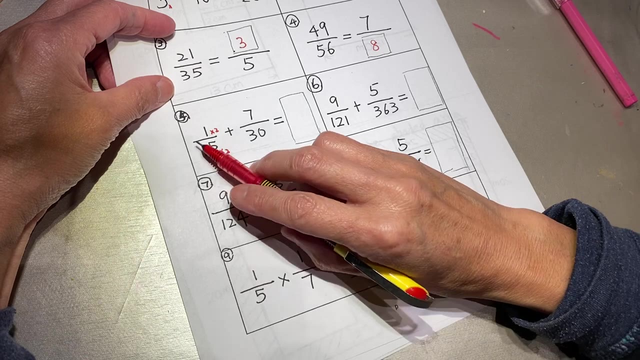 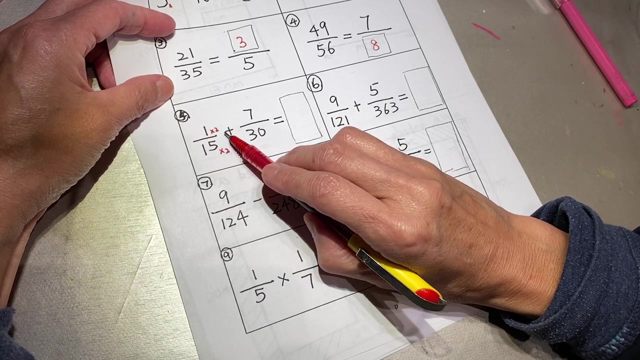 Remember, when you do fraction, addition and subtraction, never, ever, ever, ever forget the bottom will be the same. If it is not the same, make it the same. And when you time a number on the bottom, you have to time the same number on the top. 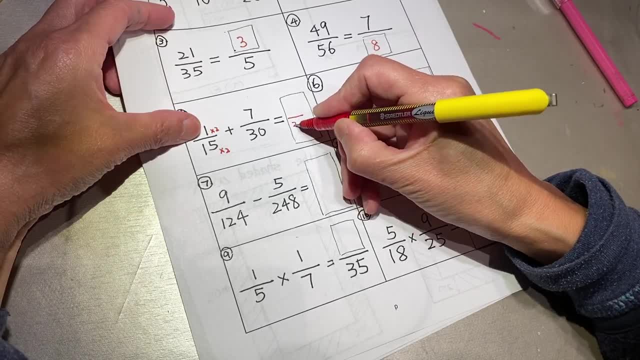 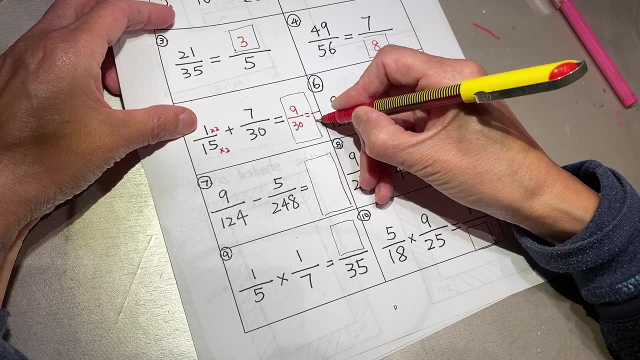 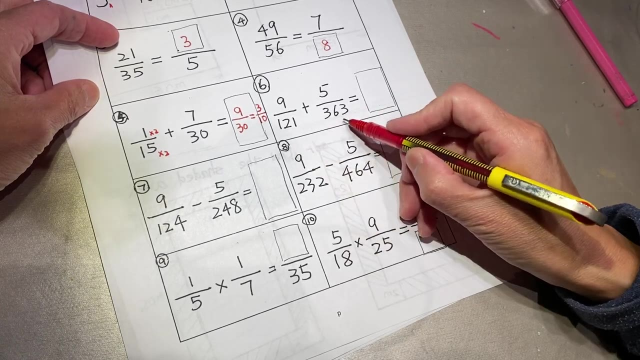 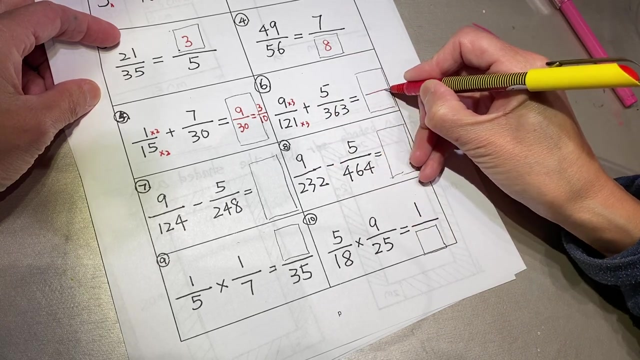 So it becomes: 30 is the bottom, 2 plus 7 is 9.. And we can simplify: It's 3 over 10.. 1, 2, 1.. 3, 6, 3.. So times 3.. Times 3.. 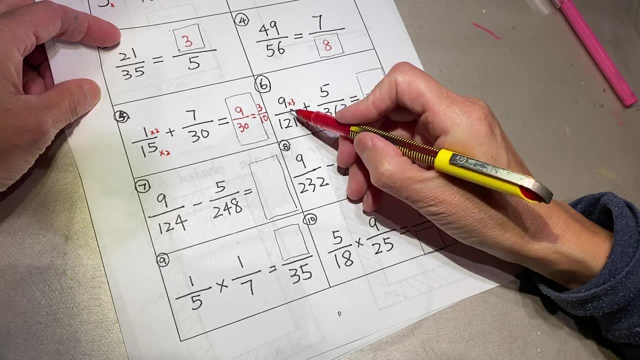 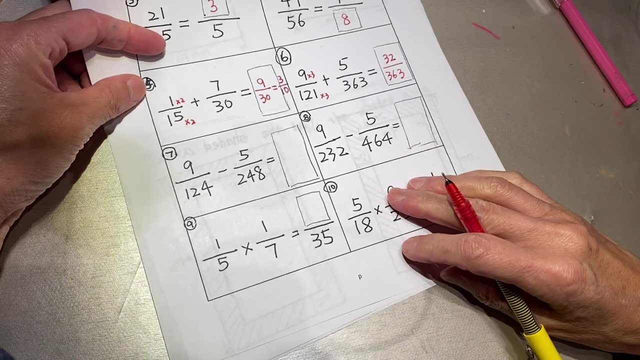 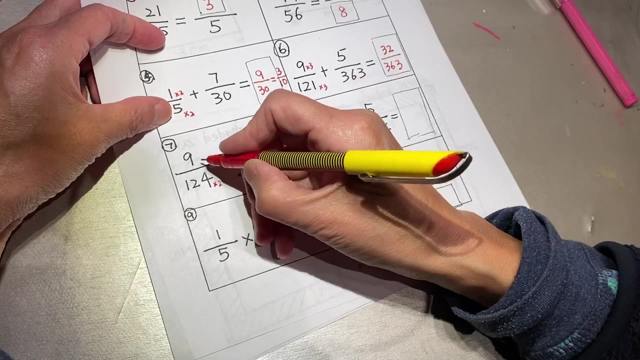 3,, 6,, 3. 27 plus 5. 32.. OK, I will start to say Chinese: 1,, 2,, 4., 2,, 4,, 8. Times, 2. Times, 2.. 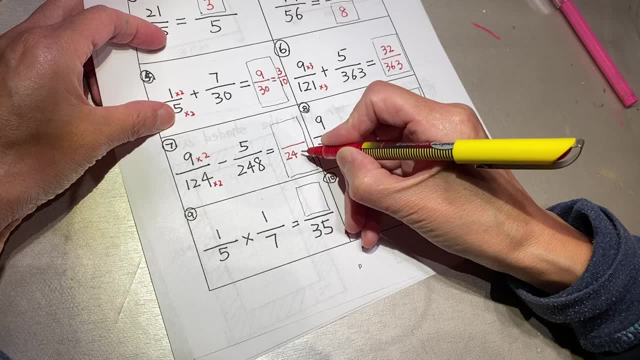 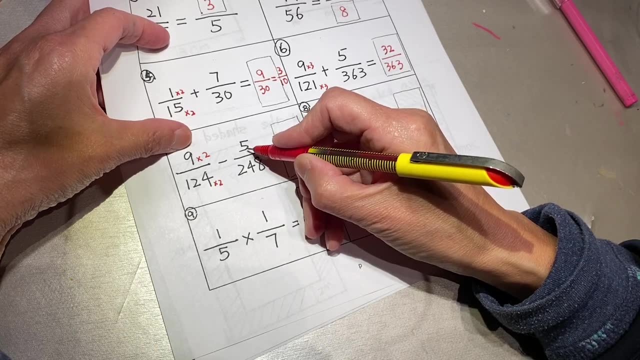 Next 2, 4, 8. Divided by 5.. 2,, 4, 8. 2, 9. 18 plus 5. 18. Divided by 5. 18.. This is divided by 5.. 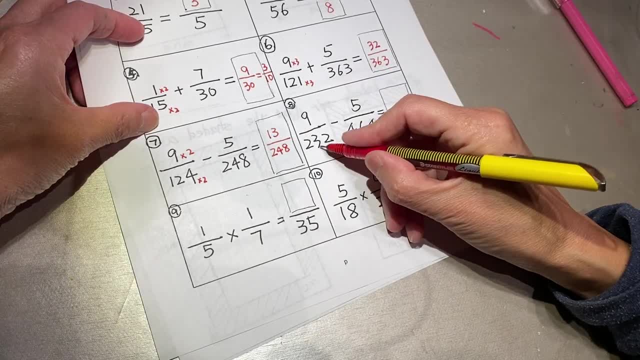 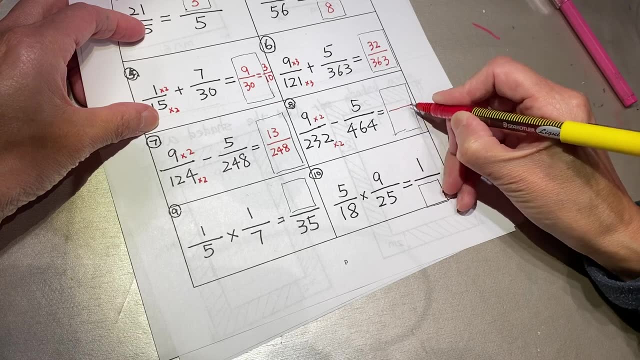 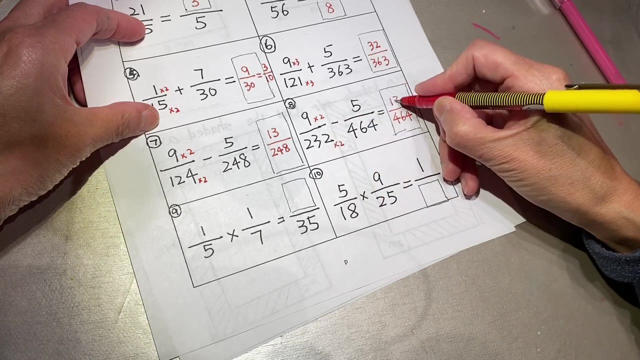 13. 2,, 3,, 2., 4,, 6,, 4. Times: 2. Times: 2. 4,, 6,, 4. 18 minus 5.. 13. The number of times. 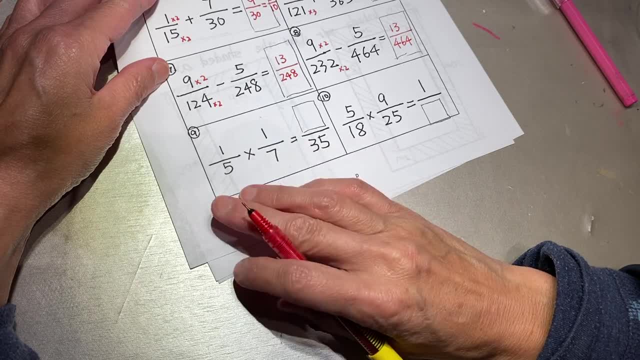 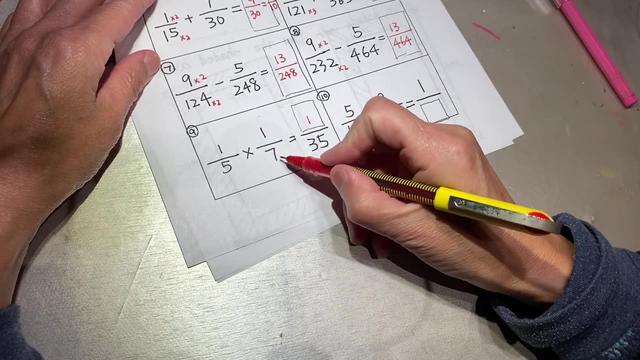 Times: The top times, the bottom, The bottom times, the bottom Times directly Times 5 times 1.. Times 1. 4 times 3.. 5 times 1 equals 1.. 5 times 7 equals 35.. 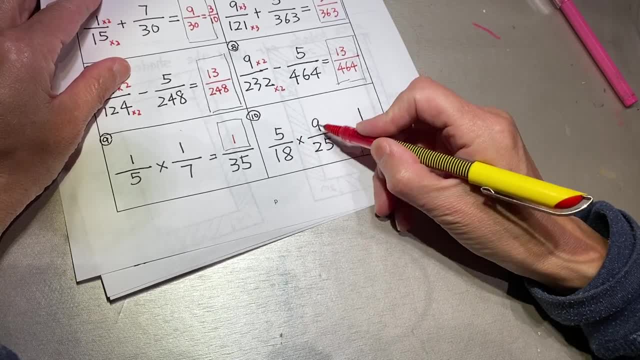 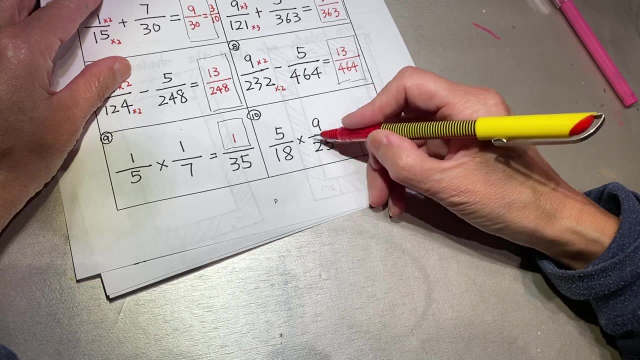 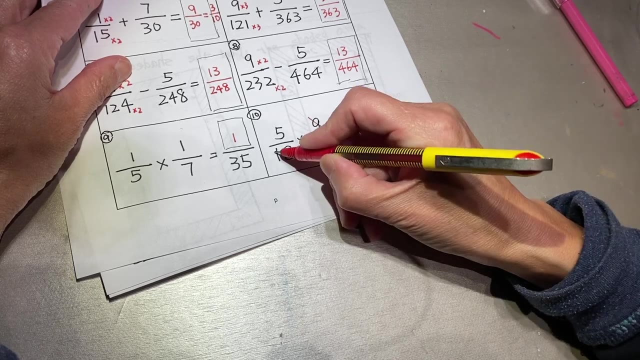 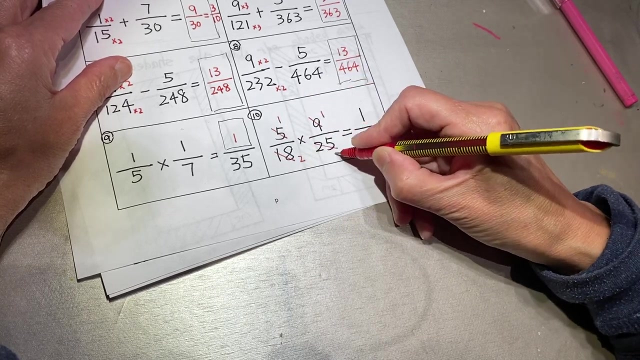 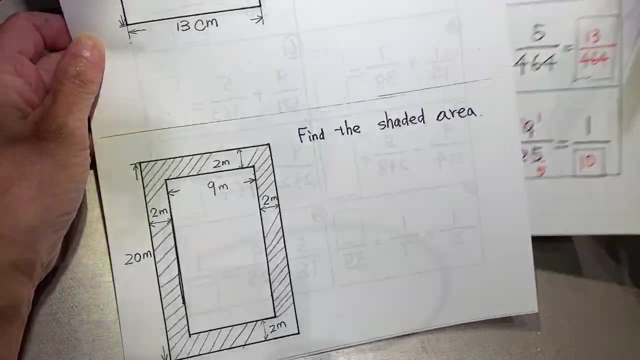 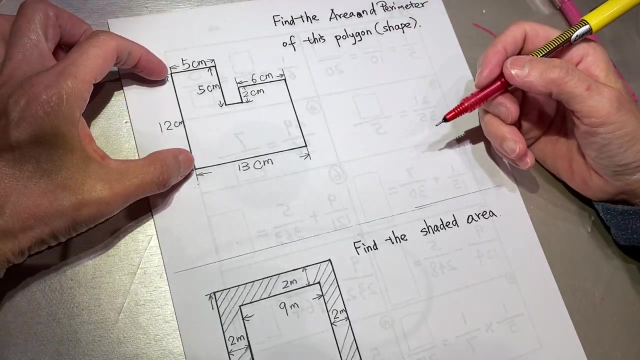 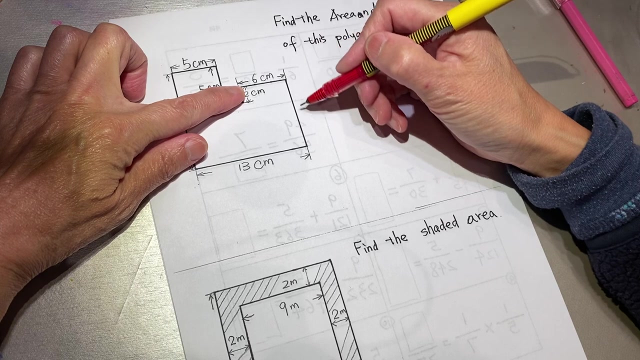 The top times the bottom. But at the same time you can check your numbers: 五, 上面一, 下面十. Find the area and parameter of this polygon: 十二, 十三, 这个是多少. 到这儿是十二. 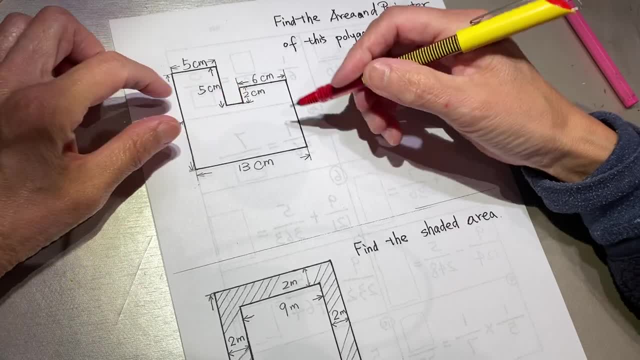 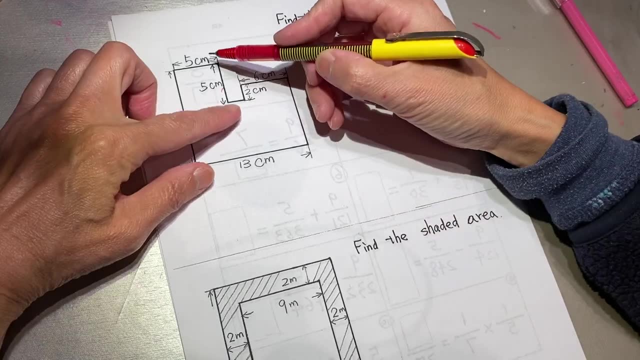 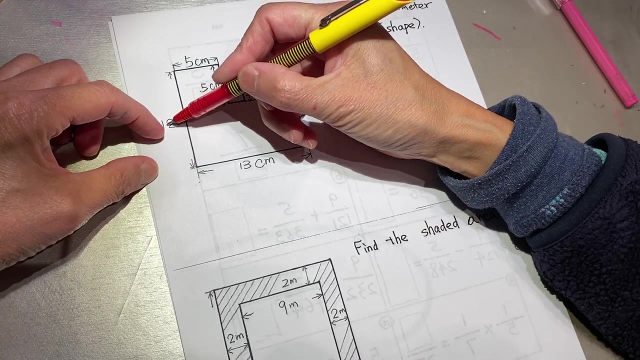 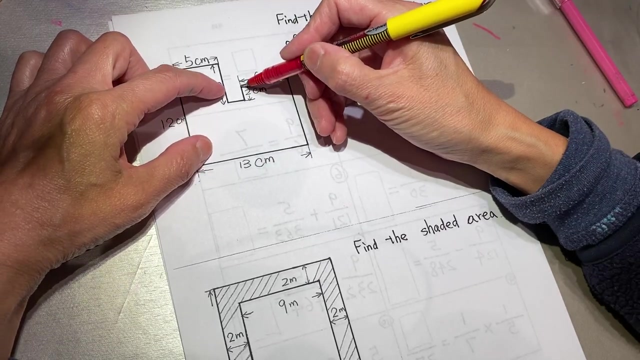 然后再加上一个二, 一个二再加上四. 这边十三 金 金, 金 十三, 所以就是二十十二加十三 乘以二再加上四. 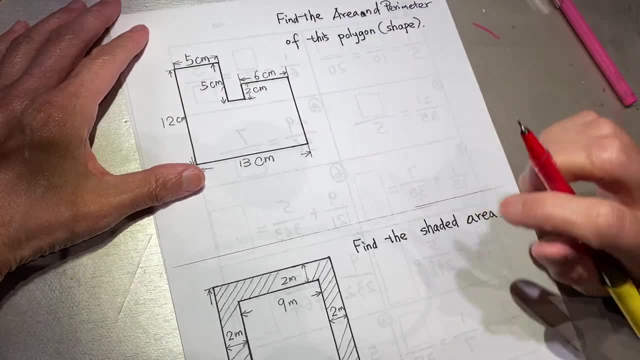 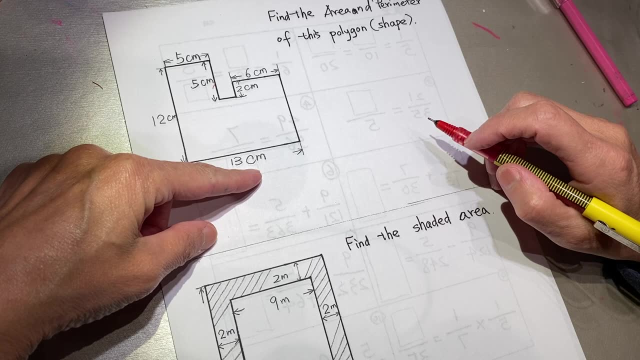 如果你看不到这一步, 我们一步一步老实算: 十二 十三 这里是多少呢? 十二 十三 这里是多少呢? 这里有二. 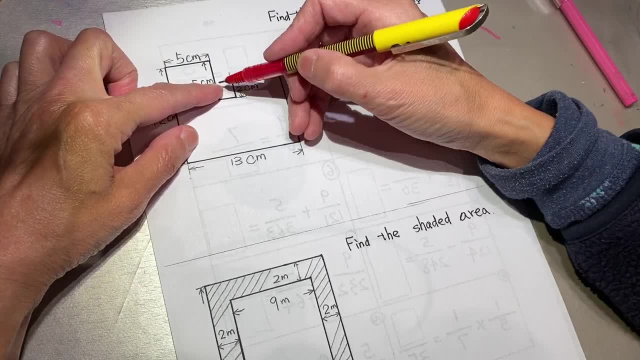 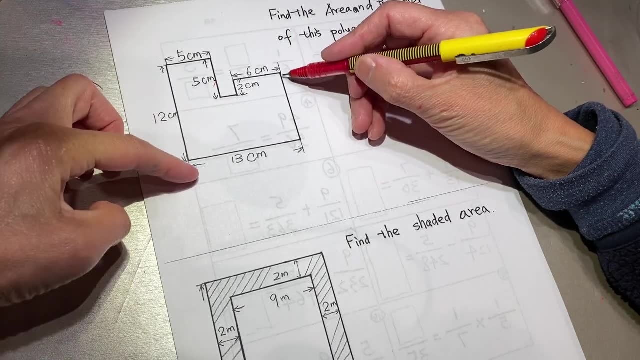 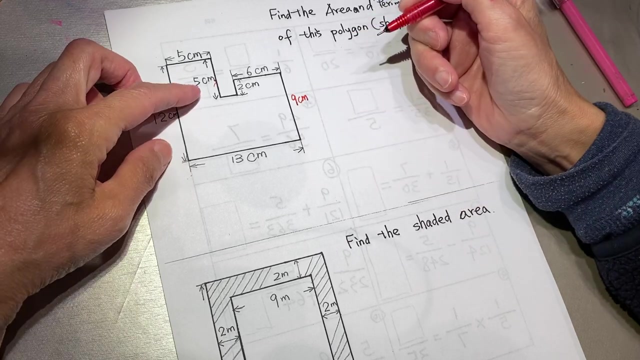 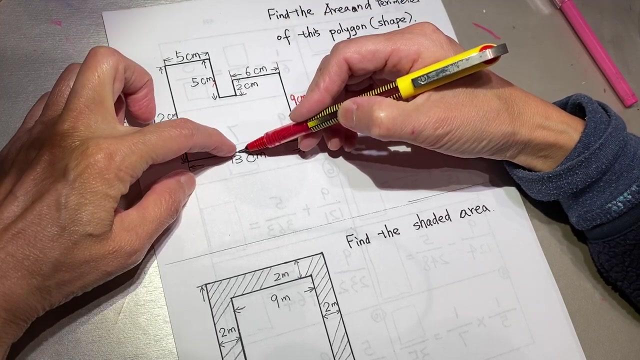 五 减二, 剩下三: 这里是三. 所以十二减三. 十二减三, 剩下九, 二减. 这里是多少呢? 十三 减五. 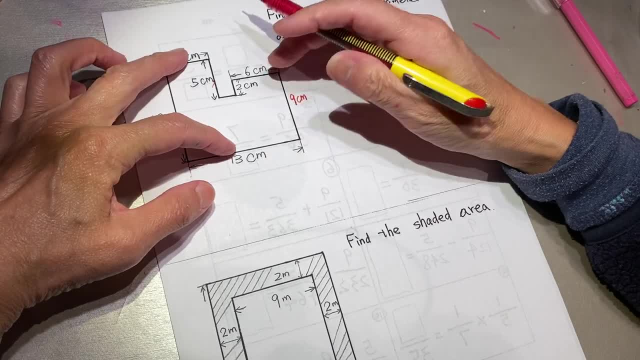 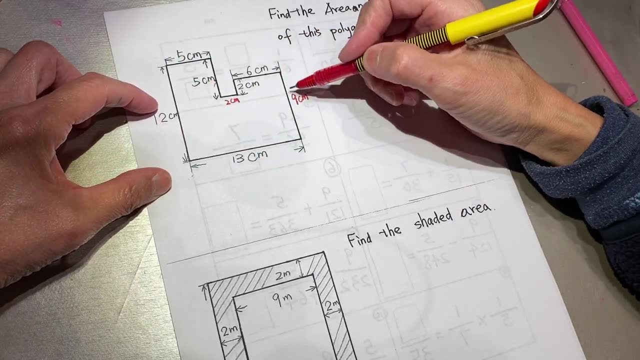 减六, 十三减五, 十一二, 十一, 二, 十一, 十一. 所以可以用这种方法一个一个加起来, 价起来, 减减, 减减, 减减. 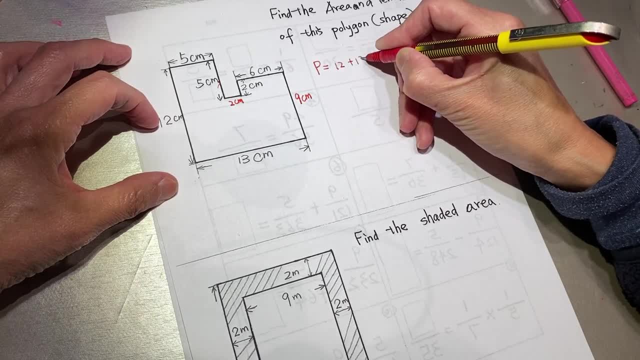 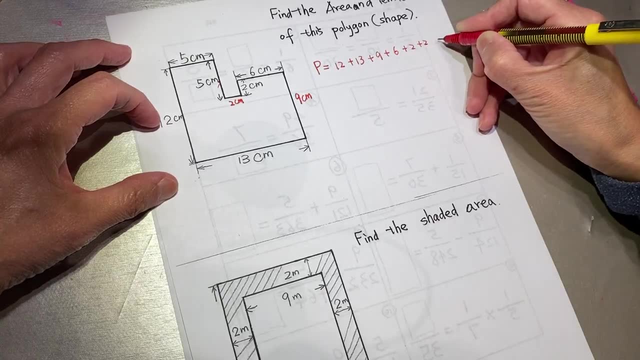 减减, 减减, 减减. 十二, 减十三, 减十三, 减九, 减六, 减六, 减二, 减二, 减五, 减五, 减五, 减五. 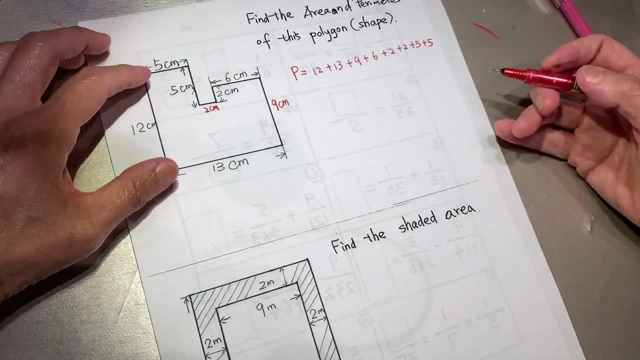 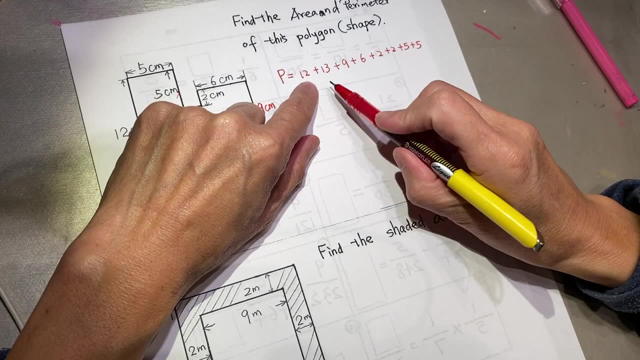 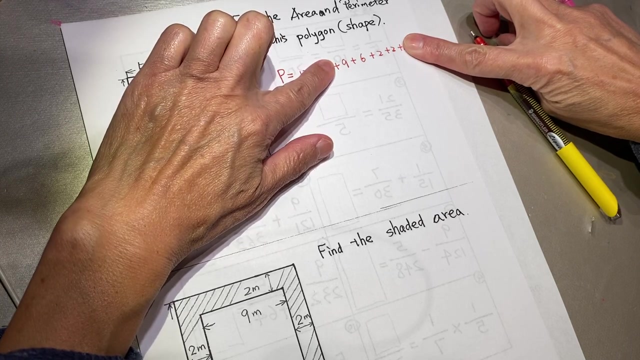 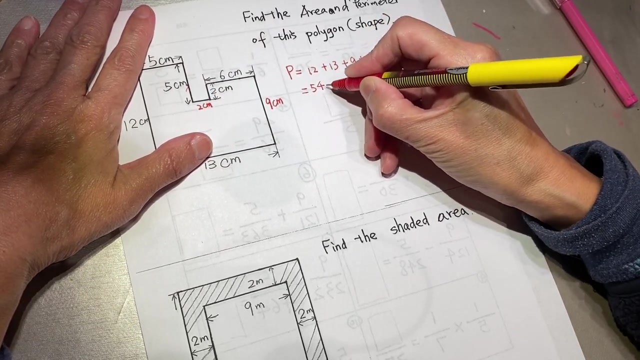 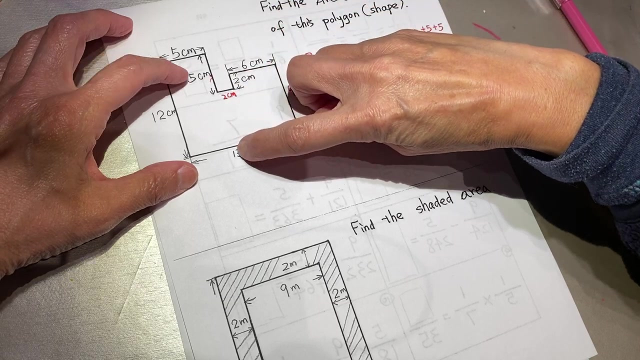 减五. The method we just calculated is 54. Let's see if it's 54 this time. 25, 35, 50, 54, 54cm. How do we calculate the area? We can divide it into three parts. 1. It's best to use a pencil to draw it. 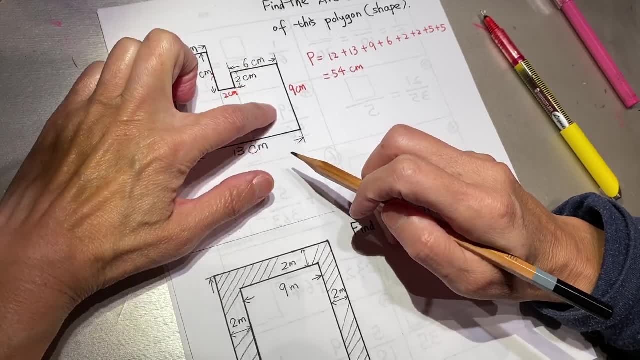 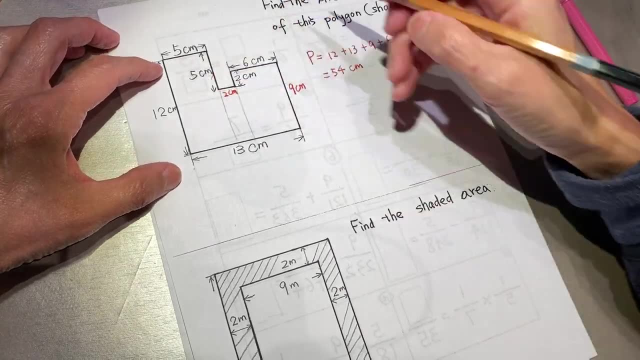 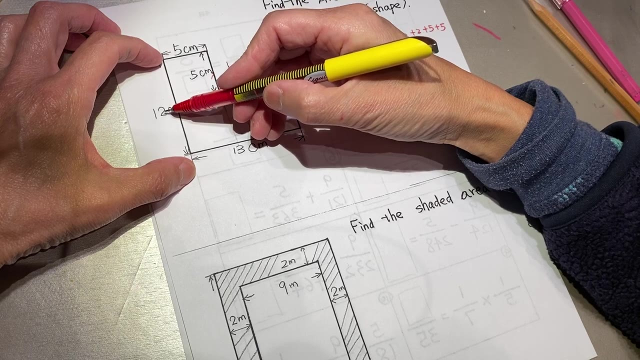 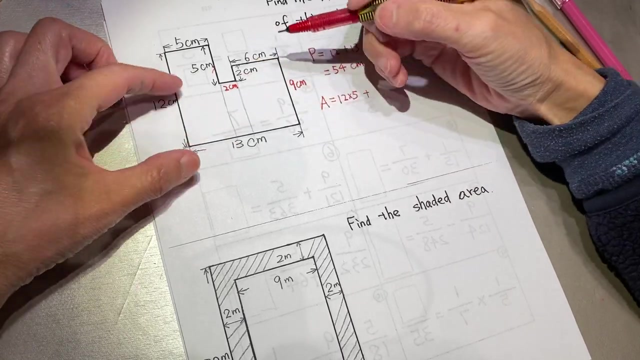 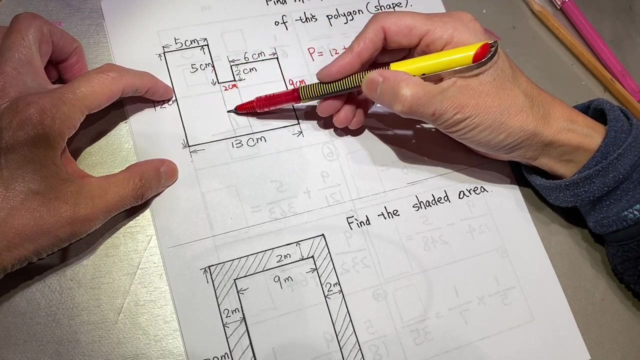 So this shape, plus this shape, plus this shape, The first rectangle, the second rectangle, the third rectangle, The first, The first, 12 times 5. The second, How much is here? Here, is 5, It's a total of 12, So the rest is 7.